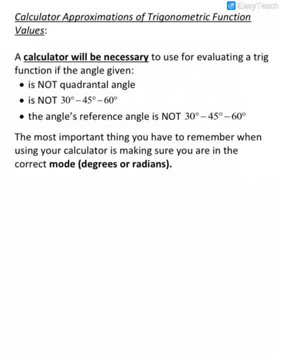 the angle's reference angle is not 30,, 45, or 60 degrees. The most important thing that you can remember when we're using our calculator is to make sure that you're in the correct mode, either degrees or radians, depending on what type. 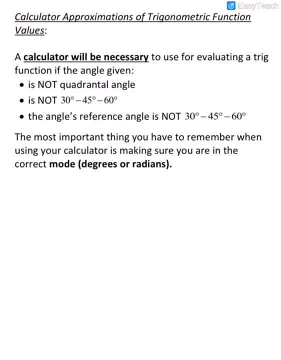 of measurement you're needing Now. the calculators that we're going to be using in finding these approximate values are the two that are allowed in this course- the TI-36X Pro or the TI-30X IIS- and I'm going to show you how to use both of those. 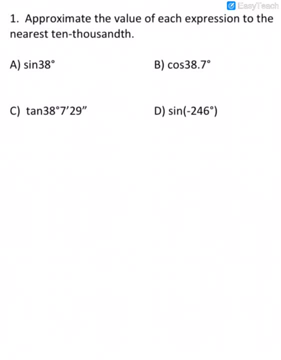 So to approximate the value of each expression to the nearest 10,000th. first of all, if we see the little degree symbol, then we're going to know that your calculator needs to be in degree mode. So to find the approximate value of each of these, I'm going to show you what it looks. 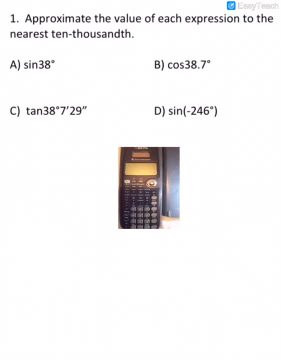 like with the camera. Okay, so this is the TI-36X Pro. If you have this calculator, let me turn it on. you need to make sure that you are in degree mode So you can see right here in the screen what mode you're in. 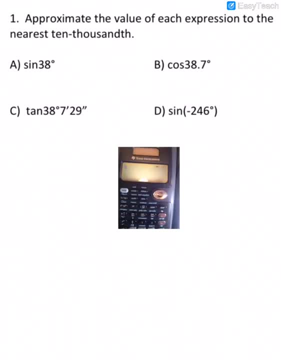 So it says that I'm in degree mode. If you were not in degree mode, if you're in radians, then you just press the mode button, which is this button right here, and you see, degree is highlighted. If it were on radians, then 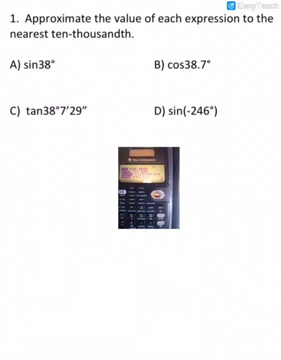 You would just scroll using the little silver scroll buttons. So this scrolls. you know, if we wanted it to be in radians, we would go there and hit enter, but we want it to be in degrees, so I can get out of that by pressing second and 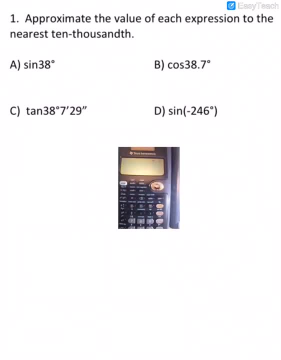 quit And then to find the sine of 38 degrees. so here are our sine, cosine and tangent buttons. So we would just press sine and then 38.. So it's in In degrees. we can close the parentheses or not. 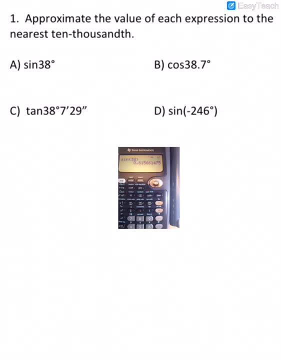 In this case it really doesn't matter, And they want us to approximate the value to the nearest 10,000th. Okay, so that would be 0.61.. So it's 156, so we need to round up, so it would be 1616.. 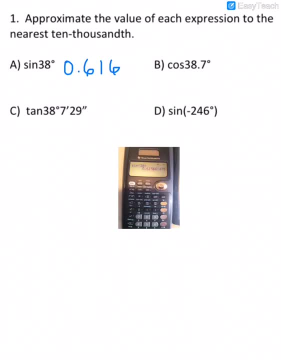 That would be the value of the sine of 38 degrees. So now for the cosine of 38.7,. I'm going to show you on the TI-30XIIS. Okay, so this is the TI-30XIIS and again on the screen you can tell what mode you're. 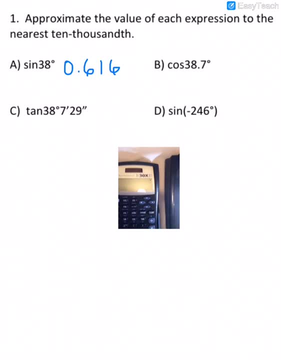 in. So if you look on the screen here- I know it's hard to see- This is actually in radians. Okay, So to change that, there is a button right here beside the second button that says DRG. So if we press that, it's on radians right now. so I'm just going to scroll over using 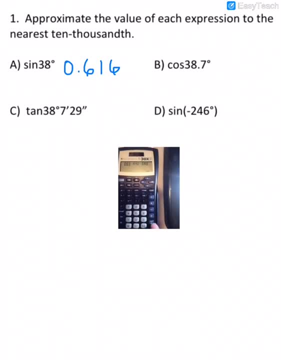 my arrows and then hit enter, hit the enter button down here and that puts it in degrees. And so now you can see on the screen that it's in degree mode. Okay, Okay, so we're going to find. We're going to find the value of the cosine of 38.7 degrees. 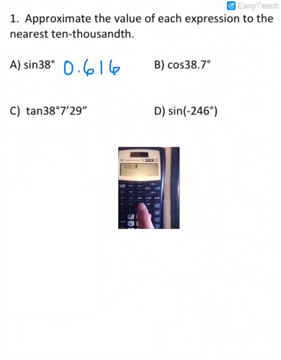 Okay, So we just press the cosine button and 38.7, and hit enter, and then again we're going to round to the nearest 10,000th. So this would be 0.7.. 0.780, because the next number is a 4, so we wouldn't round that up to a 1.. 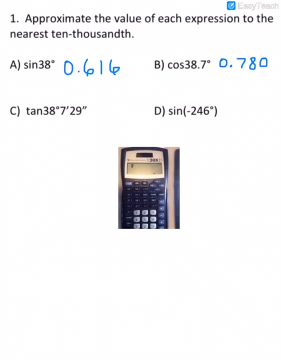 Now to find the tangent of 38 degrees, 7 minutes 29 seconds. instead of changing all of that to doing the conversion and changing it to decimal degrees, we can put it straight in the calculator And on this TI-30XIIS: if we press 10, we're going to find the tangent of 38.7.. 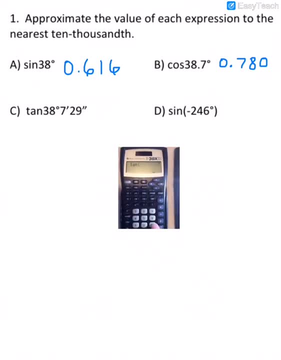 Okay, Okay. So we're going to find the tangent and then 38. There is a little button here that's got the degree mark, the minute mark and the second mark on it. So if I press it once and hit enter, that's the degree. 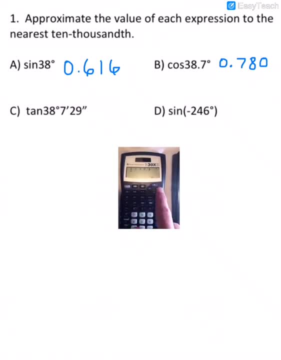 And then 7,. I press this again and scroll over. that's minutes and then 29 seconds. So I'll press it again, Scroll over twice to get to that, Okay. And then I get to the second button And I get 0.78, and then it's 47,, so that 4 would round up to a 5.. 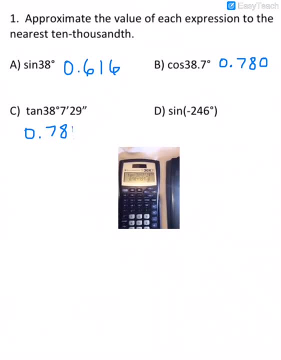 Let me write that 5 a little bit better, Okay, Okay. So let me just show you how you can do the degree-minute-seconds on the TI-30XIIS Pro. Alright, so to get the tangent of 38 degrees, 7 minutes and 29 seconds on the TI-30XIIS Pro. 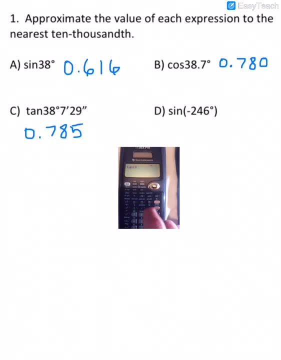 I would again just press the tangent button And then to get the degrees-minute-seconds- well, let me put in 38, then if you go to mode and Okay, Okay, Okay, Well, that's not the right thing. 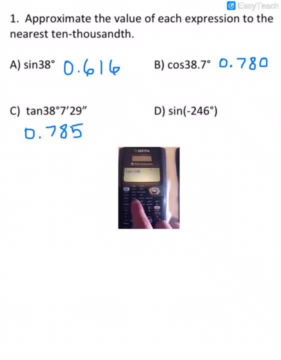 Hold on one second, Not the mode button, the math button, which is this button right here. Then we can scroll over and DMS stands for degrees-minute-seconds. so number 1 is degrees and then 7, press the math button again, scroll over to DMS. number 2 is the minutes and 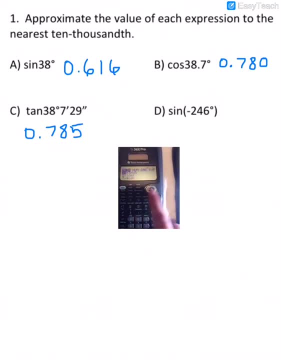 then 29. Press the math button again, And number 3 is the seconds, and we get the same answer. So then, for the sine of negative 246 degrees, let me clear this- the sine of negative. so just press the negative button. 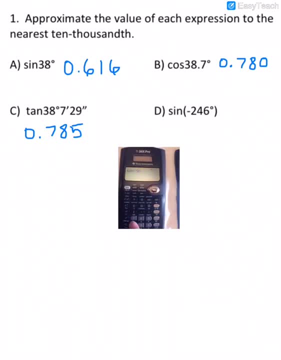 Don't press minus, because it'll come up with an error 246.. You don't have to. Okay, You don't have anything other than degrees. You know, if it doesn't have the minutes and seconds, you don't have to put the degree. 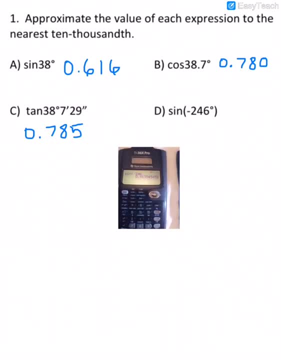 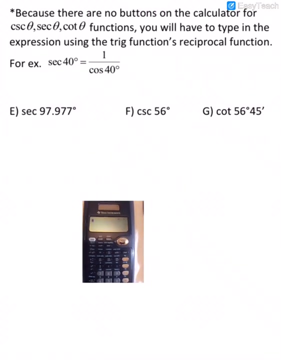 symbol, And then we get 0.91, and then 35,, so that would round up to a 4.. Because there are no buttons on the calculator for cosecant, secant and the cotangent functions. then you have to type the expression. 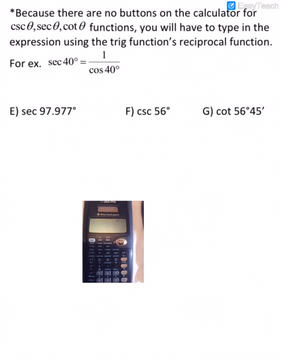 Using the trig function's reciprocal function. So, for example, if we needed to do the secant of 40 degrees, we would put it in as 1 over the cosine of 40 degrees. So for E we have the secant of 97.977 degrees, so I need to put it in as 1 over the cosine. 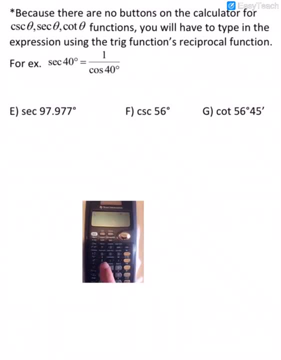 of that angle, All right. So, right here, there's a little fraction, Okay, There's a little fraction button. So if I press that button, that creates my fraction, And then, like I said, secant is the reciprocal of cosine. so well, I gotta put one first. 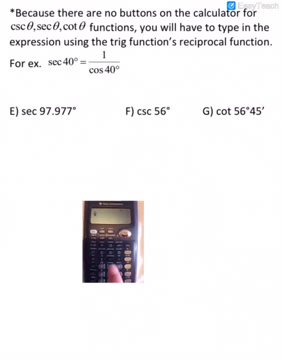 one and then scroll down to the denominator and then cosine of 97.977.. And I get a negative 7 point. What are we going to? I guess we'll still go to the thousandths place. So this would be a negative 7 point 2, 0, and then we round that to 6.. 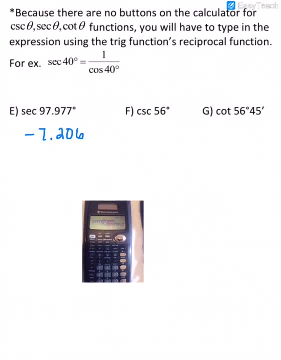 All right, So then for cosecant, let me switch to the other calculator so you can see how to do it in that calculator. All right, So cosecant is the reciprocal of sine, So we would- Um, We don't have a button that makes it look like a fraction on this calculator, so we 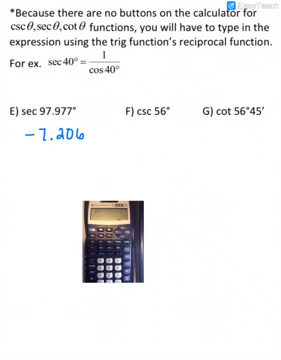 would just do 1 over, or divided by sine of 56 degrees, And just sine of 56. And then we get 1 point 2,, 0,, 6.. All right, And then for the cotangent of 56.9.. 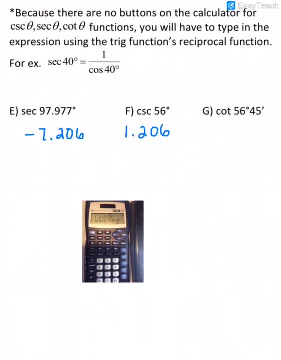 All right. So we have 56 degrees and 45 minutes. We know that cotangent is the reciprocal of tangent, So again, we would just do 1 divided by, And it would be tangent of 56.. Now, since it's got degrees and minutes, we need to put the degree symbol. 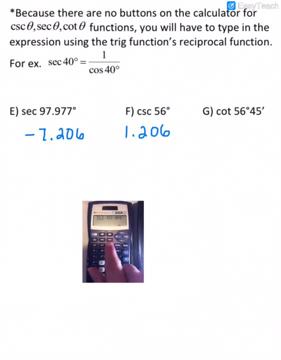 Um, Wrong thing, Let's see. Oops, Okay, So I'm going to put 45 right here, The degree symbol, And then 45 again, go here and scroll over to minutes And close my parentheses. Okay, And then I get 0 point 6.. 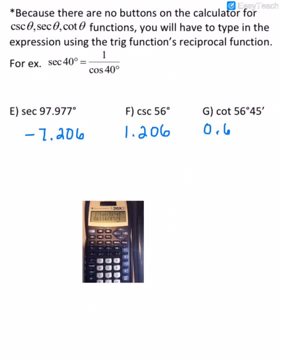 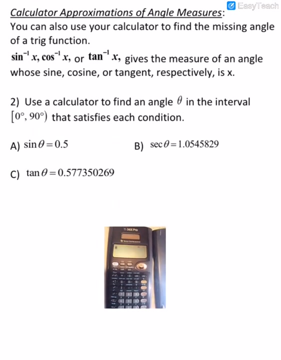 It's 6556.. So that would round up to 6.. Um, Now we can also use a calculator to find the missing angle of a trig function. So we were finding the values of the angles on the previous examples. Now we're going to find the angles for a particular value. 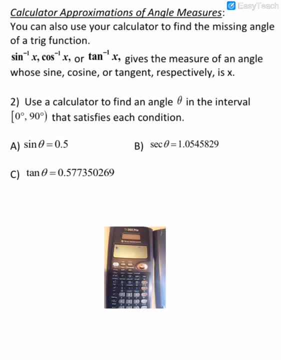 And the way that we do that is to use the inverse functions. So the little negative 1 that you see in these values here, those are not exponents, That means inverse, So that's sine inverse of x, cosine inverse of x or tangent inverse of x. 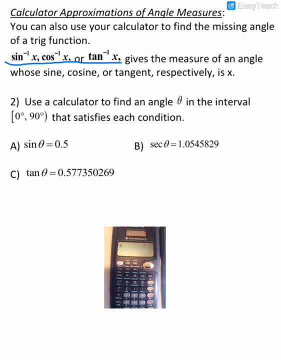 And that gives us the measure of an angle whose sine cosine or tangent respectively is x. So this says to use a calculator to find the angle theta in the interval between 0 and 90 degrees. that satisfies each condition, All right. 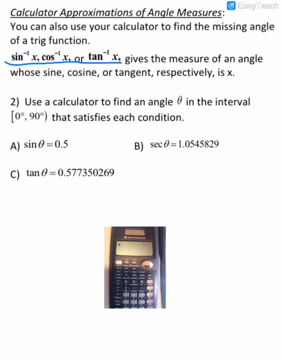 So for the sine of theta that has a value of 0.5 or 1 half, basically, what we're doing is we're trying to get the angle by itself. So to get rid of this sine off of the angle, we take the inverse of sine. 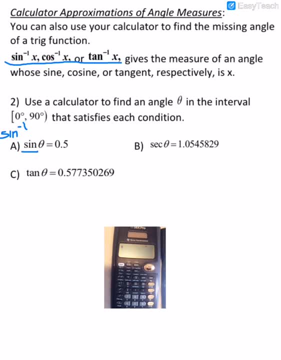 So sine inverse and sine, they cancel each other out And so we're going to take the sine inverse. Sorry about that. Let's see The sine inverse, All right, So sine inverse of 1 half. OK, So these cancel out. 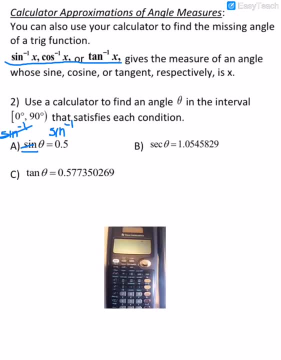 And so the angle is going to be the sine inverse of 0.5.. OK, So, if you'll notice, on the same button for sine it has sine inverse. We just have to press it twice and then that gets us to sine inverse. 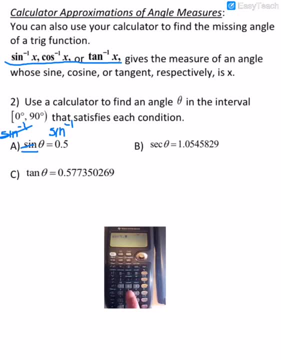 And so we're finding sine inverse of 0.5.. And that's 30 degrees. OK, So theta is 30 degrees, OK. Now for secant of theta. we don't have a button for secant, but secant is the reciprocal. 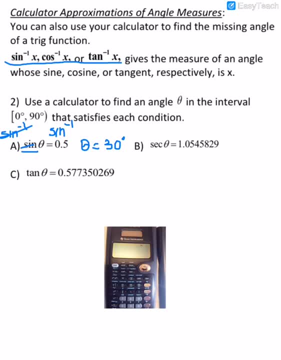 of cosine. So the way that we would put this in the calculator it would be cosine inverse. So press the cosine button twice And then we take the reciprocal of 0.5.. OK, So we get the reciprocal of the value. 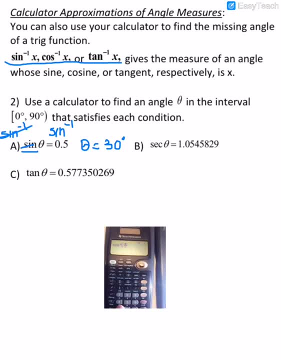 OK, So we can put it in as a fraction. So we have our little fraction button And it's 1 over what they've given us, 1.0545829.. And then scroll over to get out of the denominator And we get 18.55.. 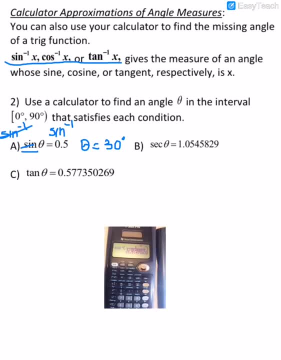 All right, 0.5 degrees for theta. all right, okay. and then for the tangent of theta, we just do its reciprocal, I mean not the reciprocal, the inverse of tangent. okay, so tangent, if we press it twice we get tangent inverse and just put in what they've given us. point five, seven, seven: